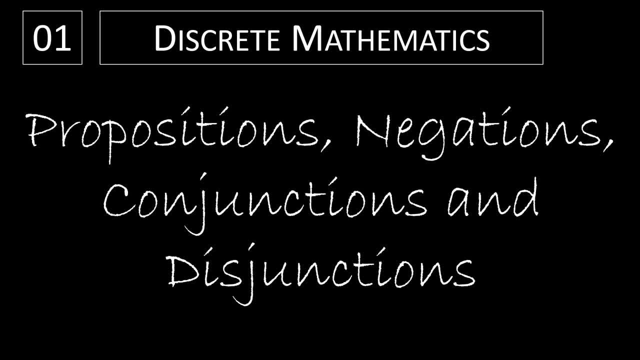 In this first video of the Discrete Mathematics playlist, we are going to look at propositions what they are, and then look at negations, conjunctions and disjunctions, And we'll also take a look at the truth tables that go along with those connectives. The connectives: 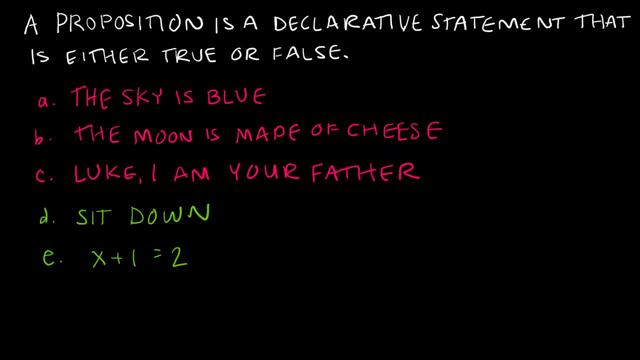 are the negations, conjunctions and disjunctions. So our first new terminology here is a proposition, and a proposition is just a declarative statement. that is either true or false. So notice: I have five statements written down. Three are in pink, two are in green. The statements written in pink: 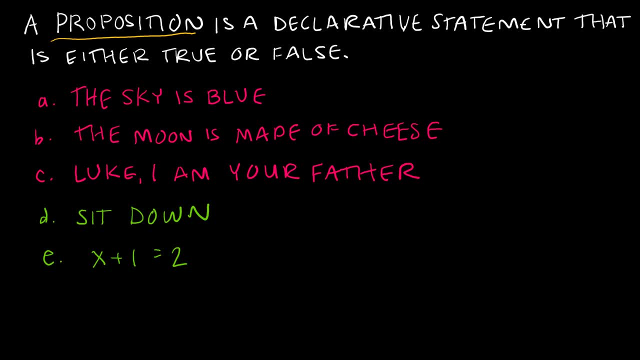 are all considered propositions because they are declarative statements that are either true or false. The sky is blue is a declarative statement. Generally, what we will do is we will take this statement and we will say: let's let P represent that. Or the moon is made of cheese, also a declarative statement. Again, that could be either true or 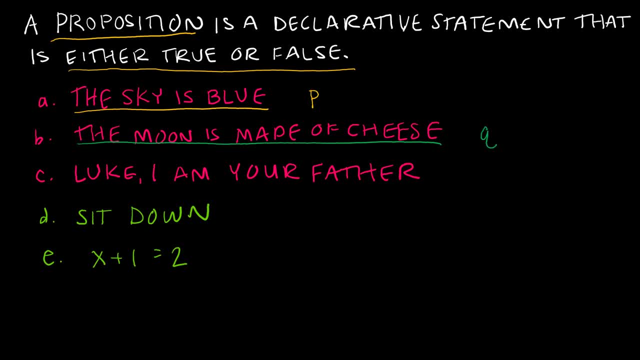 false. I'm going to say false on that one And I'm going to say that is proposition Q. The moon is made of cheese. Again, it is considered a proposition because it is a declarative statement. that is either true or false. Same thing with Luke. I am your father. This is a. 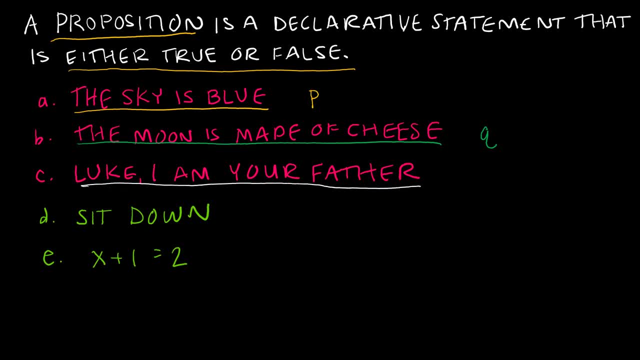 declarative statement. I am your father- either true or false. I'm going to say that one, That one's false And we'll say that's R. Now take a look at the difference of the statements that I've written in green. D says sit down. Sit down is a statement, but it is neither true nor 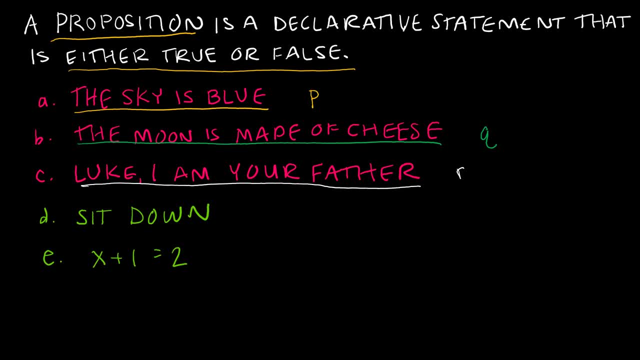 false. I can't say true, you have sat down. That statement would have to be: you sat down. That's either true or false. But sit down is just telling you what to do And that is not a proposition. A lot of people 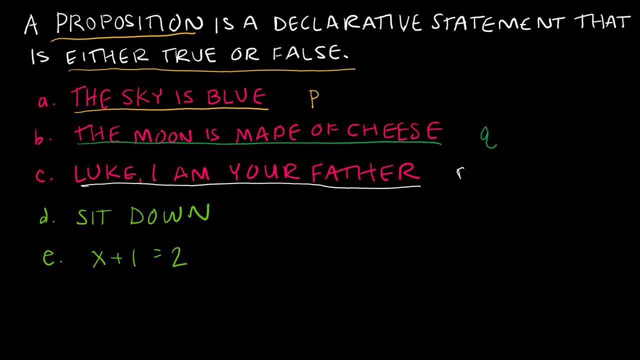 struggle with E because they say: well, that could be true or false. And while your thinking is correct, the way that it is written right now is not a proposition. If I replaced X with some value, or if I said, where X equals five, well, now it's a proposition because I can say: 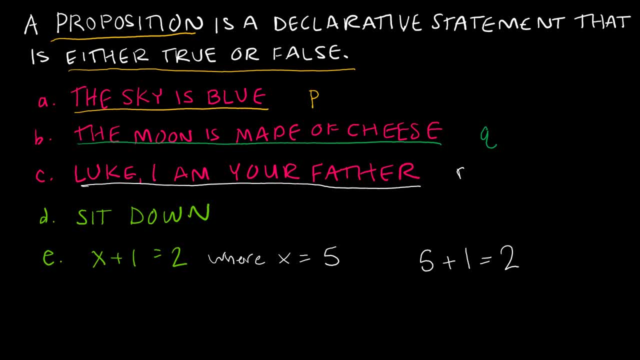 five plus one equals two is false. Or if I said where X equals one, then one plus one equals two is true. But if I don't assign a value for X and I just leave it as X, then this is not a proposition, because this is not true or false. So propositions themselves are fairly straightforward Again. 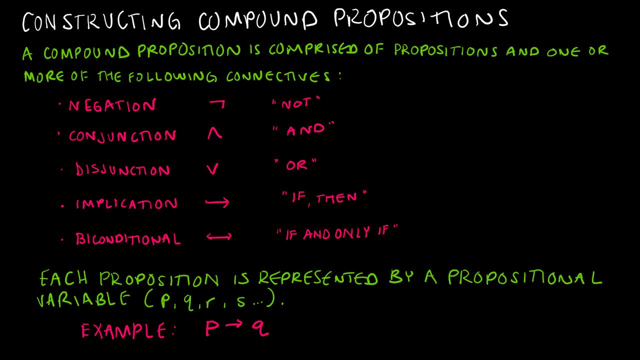 we're using a lowercase letter- PQRS, et cetera- to represent a proposition, And then what we're going to do is we're going to end up making a compound proposition using these connectives. So I want you to think of these connectives. 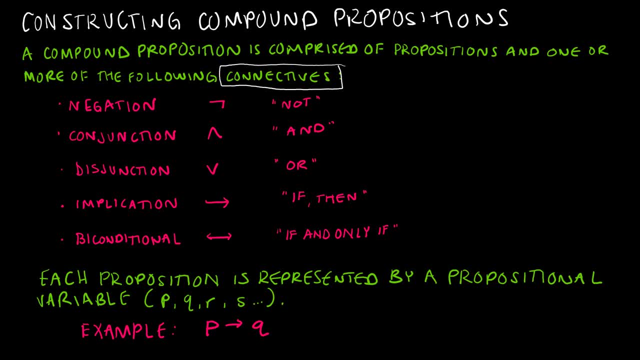 operators, as I would take one plus two. That's an operator, So these are just operators for propositions And I've put them all on one page together, just to have one page that you could refer back to. They're all called connectives, So we're going to go through each of these in. 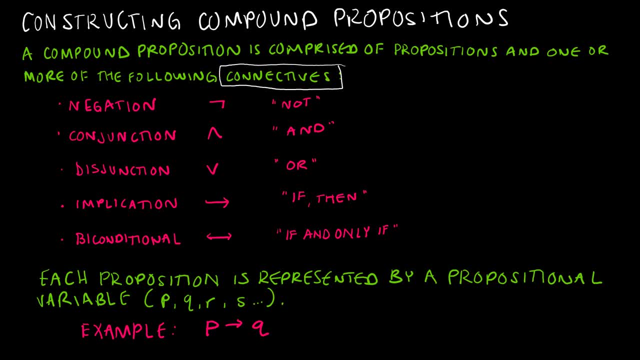 detail in the following slides, but I did want to put them all here, So let's talk about them very quickly. We have the negation, And again this is how we would use that negation. So I would say not P, And again I would say it as not, but that is the symbol that I would use. Conjunction is: 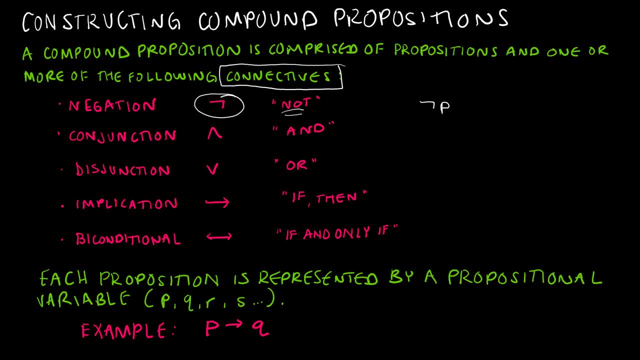 and And again. we'll talk about each of these in detail. So obviously I would be taking P and Q. A disjunction is an or, So that would be P or Q. An implication is an if, then. So this is an if P. 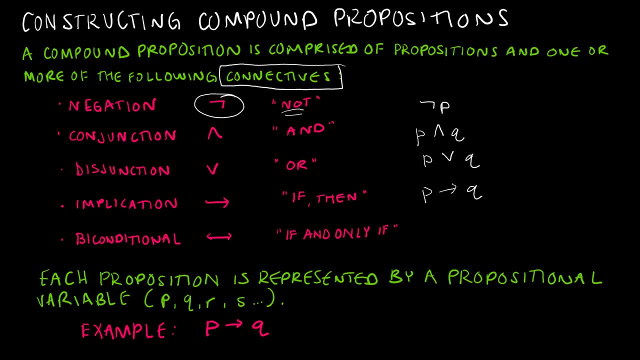 and Q, And then a biconditional notice. it has an arrow on each end here says if and only if. So P, if and only if Q, And that means they both have to share the same truth value. So again we're using P, Q, R, S, et cetera, using those lowercase letters to represent 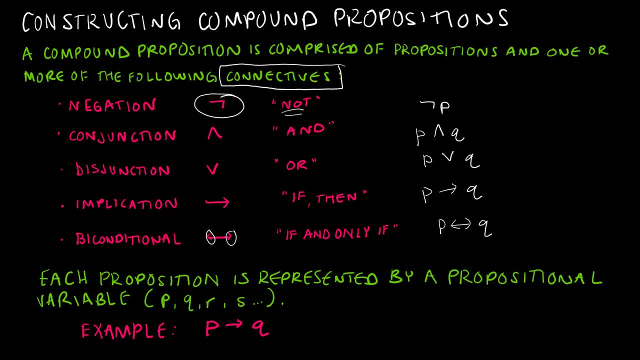 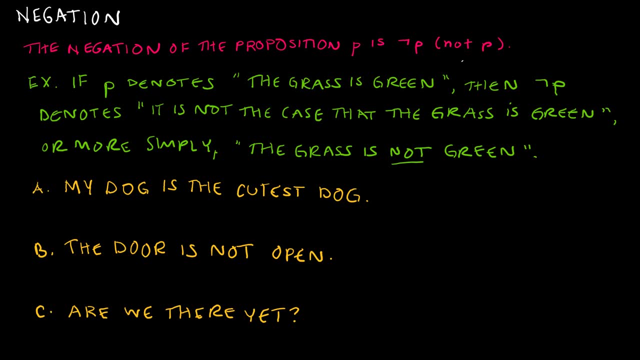 each proposition. So let's get into each of these connectives in further detail. The first connective is a negation And again the negation is not, And this is the symbol that we would use. So the negation of the proposition P is not P. So example, if I say P denotes the grass is green. 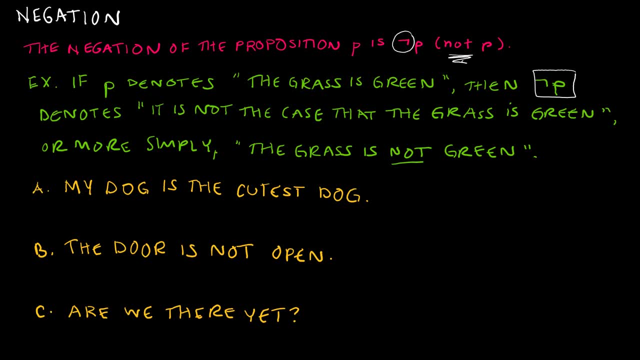 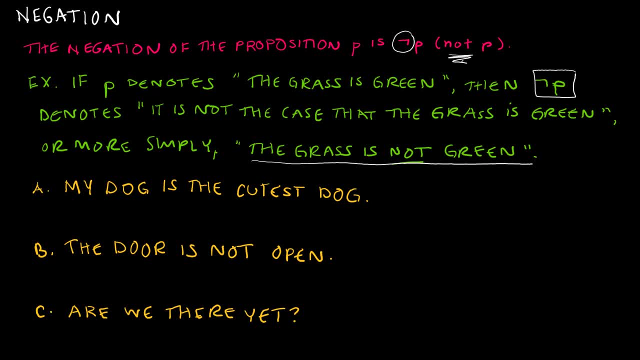 green. so let's take a look at these few examples I have here, and then I want to look at some truth tables with you to make sure that this all makes sense. so the first one says: my dog is the cutest dog, which- this is a true proposition by. 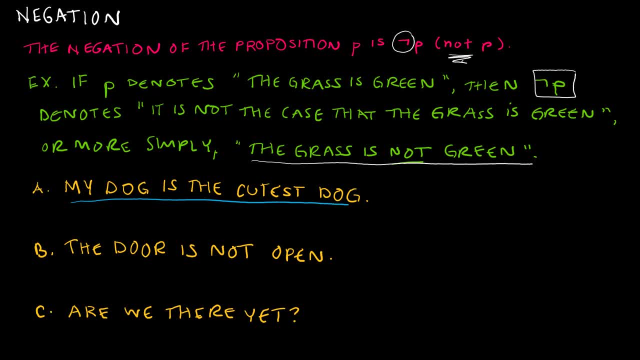 the way. so my dog is the cutest dog, is my proposition P? if I want to write not P, then it would be my dog is not the cutest dog, so that is not P. again, we could say it is not the case that my dog is the cutest dog, but it's easier to. 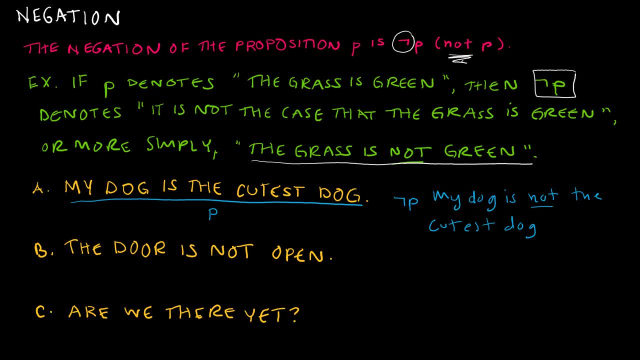 write it the way we would normally say it in the English language: the door is not open, is not open, is P? now again, if the door is not open, is P then if I'm negating something that already seems like it's negated? remember, in mathematics is the only place that 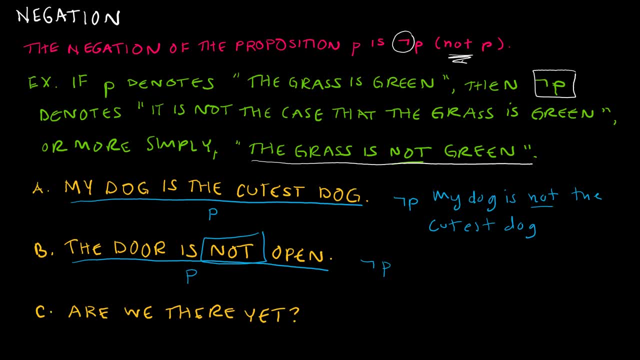 two wrongs do make a right. so the door is not not open, which means the door is open. again, we could say: it is not the case that the door is not open, but in real life we would just say the door is open. last one: are we there yet? be careful with this, because this is not a 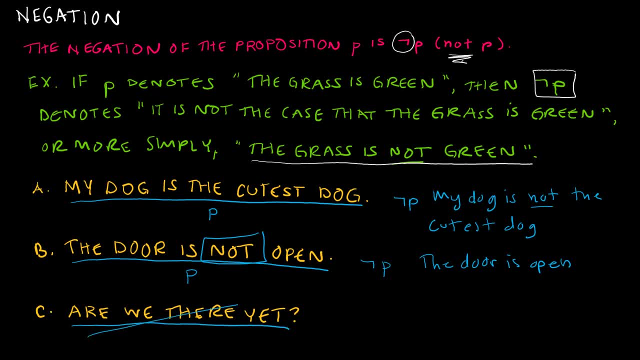 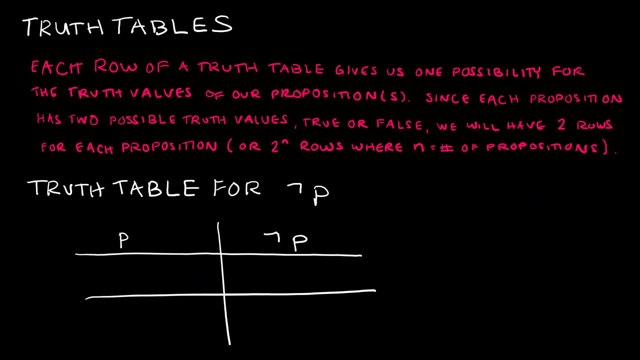 proposition. it's not a declarative statement. that is either true or false, and because of that I can't negate it. so let's talk now about truth tables and how a truth table works. so if we have a truth table, essentially what we have is a row for each possibility of the truth. 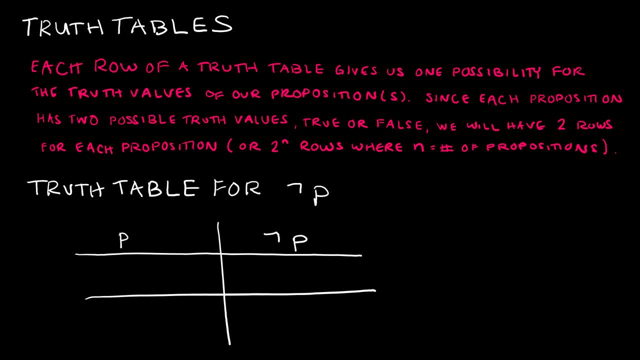 values of our proposition. so I want you to think of this as a as having two parts. so this is a very, very basic truth table that we're going to do, but the left side of our truth table has all of the combinations of the truth values for our propositions. so in this case, if I just have one proposition, 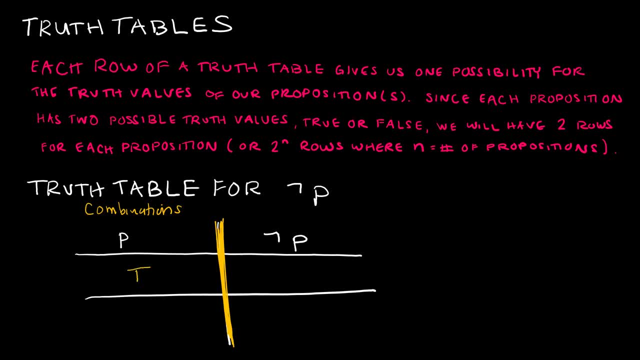 P. that P can either be true or it can be false. so let's say P again represented my dog is the cutest dog. then not: P represents my dog is not the cutest dog. so how does the truth table work? well, again, on the left side, we're going to give all of the 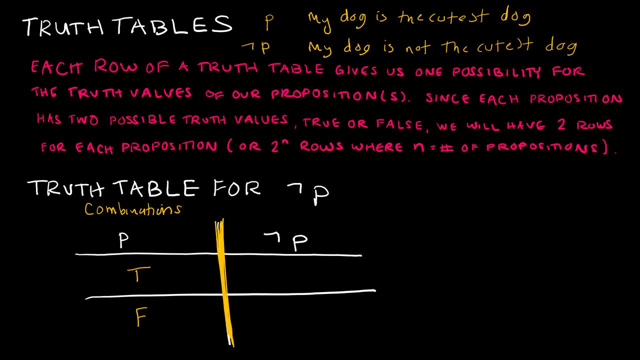 combinations, which is very easy for one proposition, and on the right side we're going to use whatever our connectives are, and so we might have several columns on each side. in this case, we just have one column on each side, but we might have several depending on how complicated our 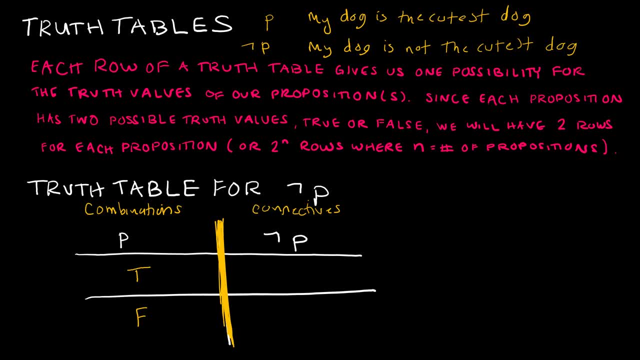 truth values or truth table is going to get in this case. let's look at our proposition P, and here's how a truth table works. let's say: P is true. so here I am. P is true, my dog is the cutest dog is a true statement. 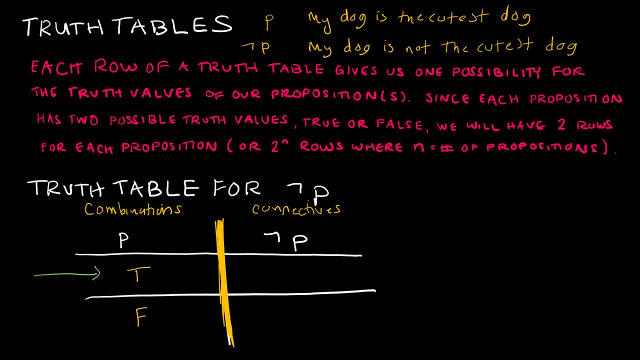 which means not P, my dog is not the cutest dog, would have to be false, because my dog can't be the cutest dog and not the cutest dog at the same time. let's say instead that my proposition was false. I said my dog is the cutest. 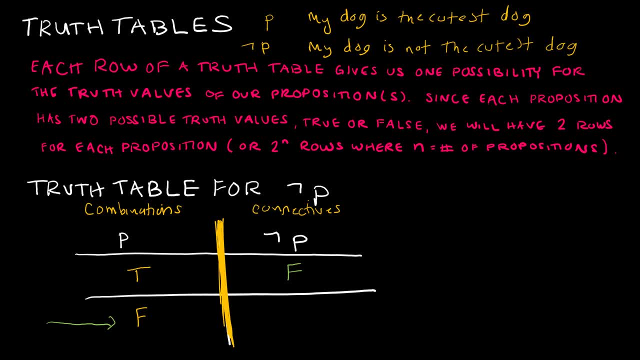 dog and that is an incorrect statement. then not P, which says my dog is not the cutest dog, would have to be a true statement. so that's how it. truth table works is on the left side. we have all of the different combinations. on the right side we have whatever connectives we're going to use. 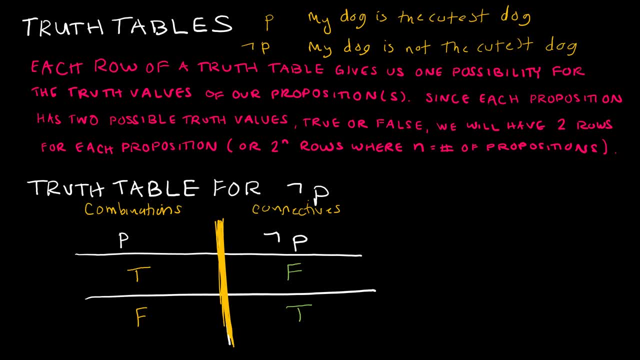 truth, tables are going to be very important to us, so that's why I wanted to introduce them to you in this video, so that you had a good foundation when we get to our next video, where we're going to use them in more detail. before I continue on to our next proposition, I just want to remind you that in this 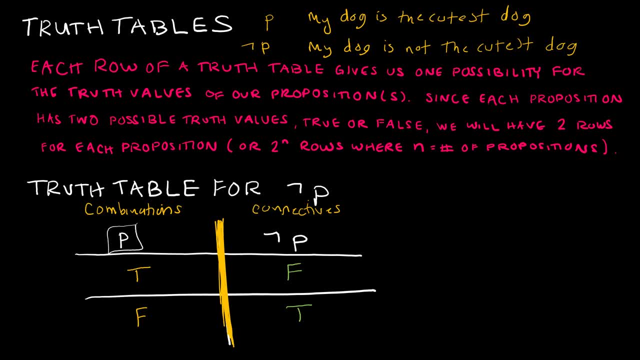 case, I only gave you one proposition. we're going to have several, in fact, our very next example is a proposition where I have to, or, excuse me, a connective that requires us to use two propositions. so if I have two propositions, I'm going to have two to the N rows, which is two squared rows. 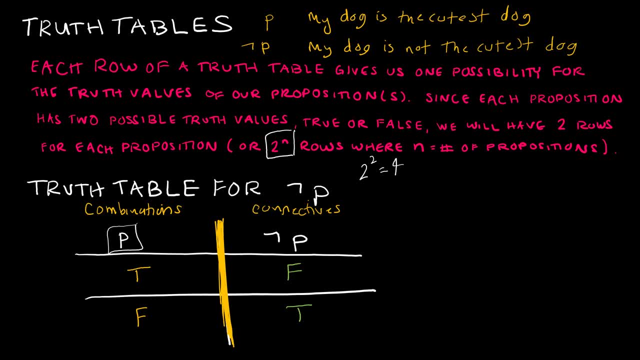 or four rows, and really this is all about just how many combinations are there. let's say, I'm using P and Q and it doesn't matter what the connective is in between there, so we're going to do P and Q, we're going to do P or Q and we're 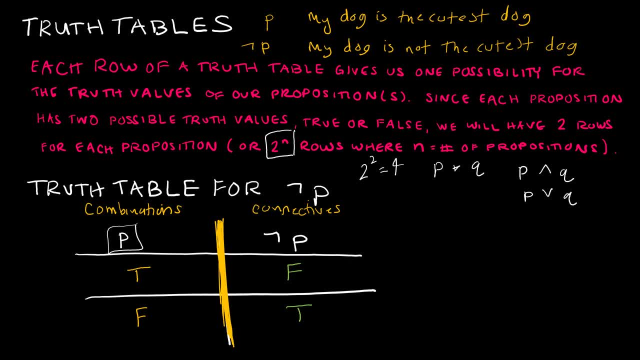 going to do these in just a little bit, but just so we understand. the left side would have to have all of the values for P and all of the values for Q, all of the combinations of those two. so here's the best way to go about this. if I've got P, 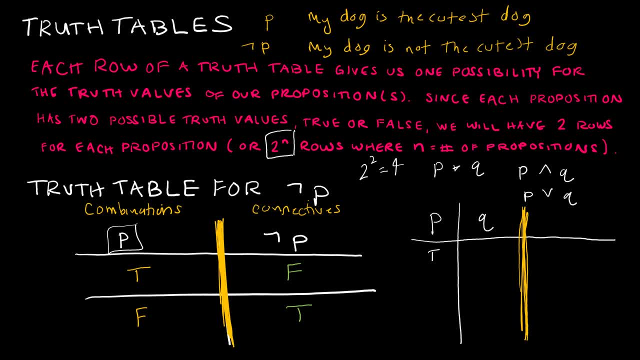 and Q here, then P could be true and P could be false and P could be true and P could be true and Q could be true. P could be true and Q could be false. then it's also a possibility that P is false and Q is true, or P is false and Q is false. so 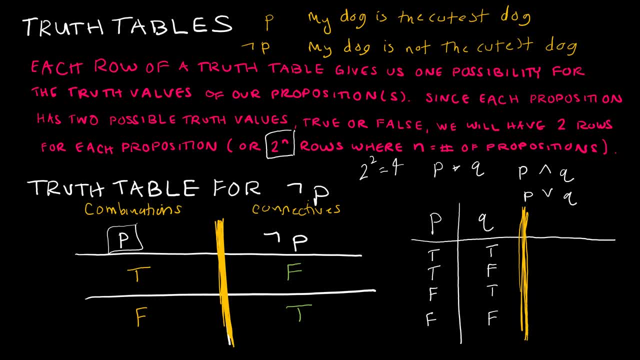 notice on the left side which has two columns. these are my combinations. now do your professor a favor and write them in this way. I have a lot of students who do true, true and F as, because P and Q are both correct, poisoning, and Q is false, and then false, true and then false, false, true, false, and it gets very hard for me. 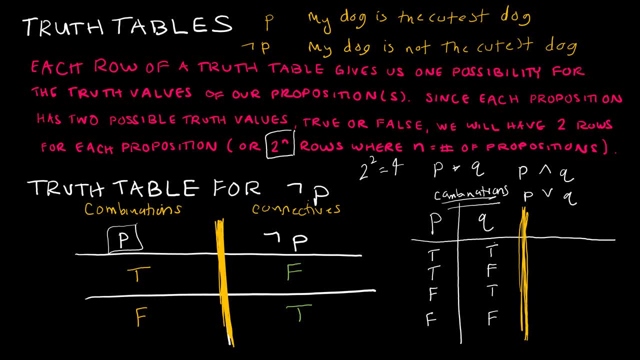 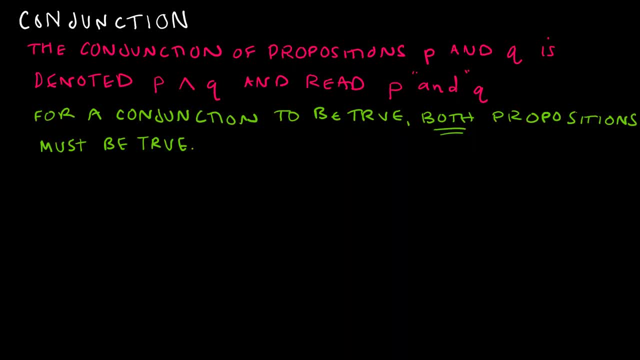 to check your work when you're all willy-nilly like that. so do me a favor: keep these grouped together, and then these will alternate and we'll continue to work on that together. our next connective is called a conjunction, and a conjunction of propositions P and Q is denoted P with the little arrowhead. 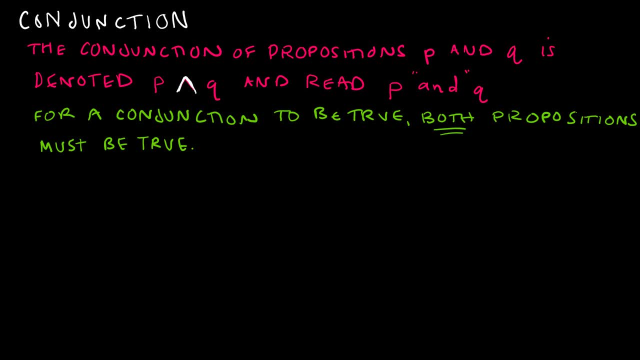 basically Q, and it's read P and Q, so a conjunction is an, and, and one way to help you remember this is: this kind of looks like a capital A if you added that little marking in the middle. now, the reason I bring this up is because our 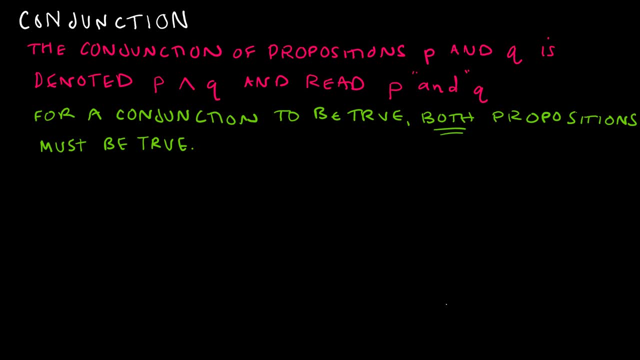 next one is going to be the arrow pointing down instead of the arrow pointing down, and the next one is going to be the arrow pointing down pointing up, so it's good to be able to keep them straight. for conjunction to be true, both propositions must be true, so we're going to create the truth table. 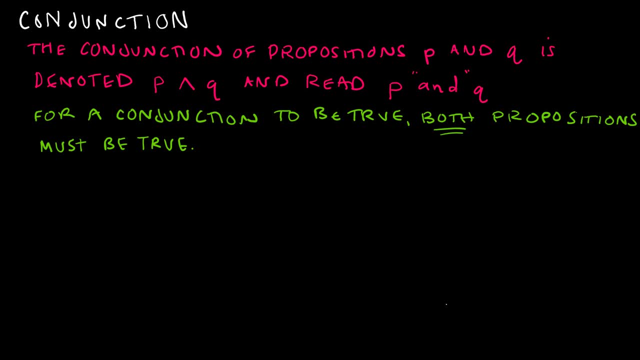 together. but it's also important to think about the fact that P and Q represent statements. so let's say P is it is raining, Q is I am arep, Compl, crushed. wait a second. say that again, just as a, because it was a. closed captions can't treat them as pleb. in any case, that's the so useful English meaning that I used to C. you know I might understand Thurman and what's if you have. whether it's you hear the characters. 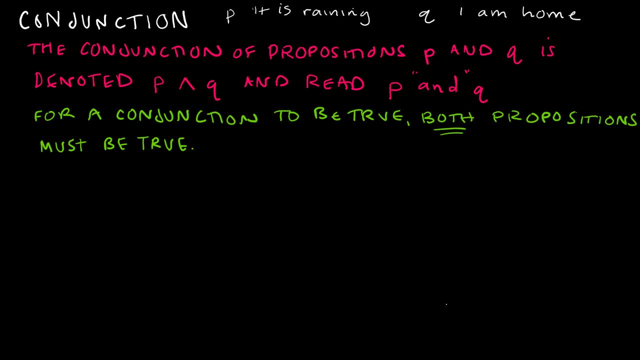 home. So if I'm creating my truth table, remember there are two sides to this, And on the left side is where we just give all of the different possible truth table combinations And since there are two propositions, that means it's going to be two squared or four different rows. So I'm 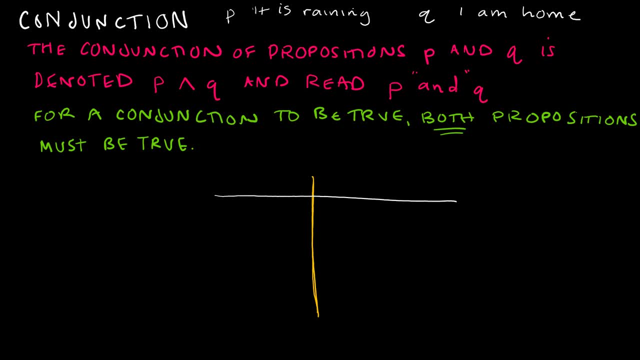 going to. this is not going to be a row, This is just going to be where I put my values P and Q. So I need four rows, So one, two, three, four rows And, of course, a column for each of my. 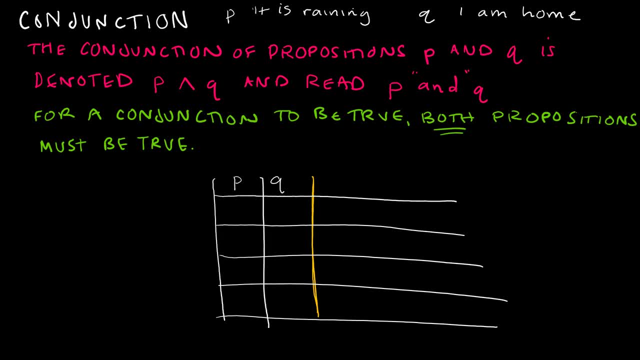 propositions. So I've got P, Q and I'm going to list all of the combinations. So P could be true with Q, true or true, false Or false, true or false, false. So that's all of the combinations. On the right side is always going. 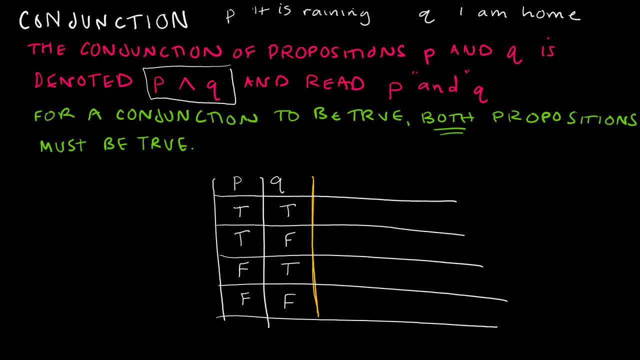 to be whatever it is that you are doing, a connective of. So in this case, we're only doing P and Q, or the conjunction of P and Q, And that's the only thing I will need on the right side of my truth table Now, before we start filling it in, let's think about what this means. So I'm going. 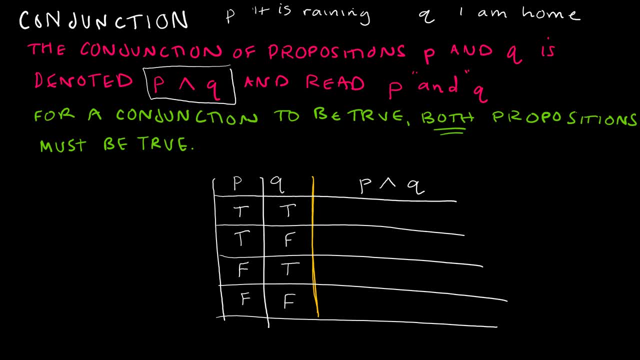 to look at the two propositions. P says it's raining, Q says I'm home. For this conjunction to be true, both propositions must be true. So it must be raining and I must be home. So this says P is true, Q is true, It is raining and I am home. The only way for P and Q to be true is for both P and Q to 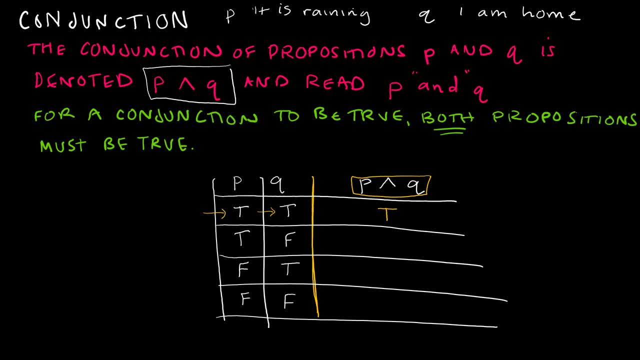 be true, And that is the case here, True, true. So P and Q is true. For the rest of the rows: this row represents it is raining. I am not home. So that's false because they're not both true. because I'm not home, This row represents it is not raining. 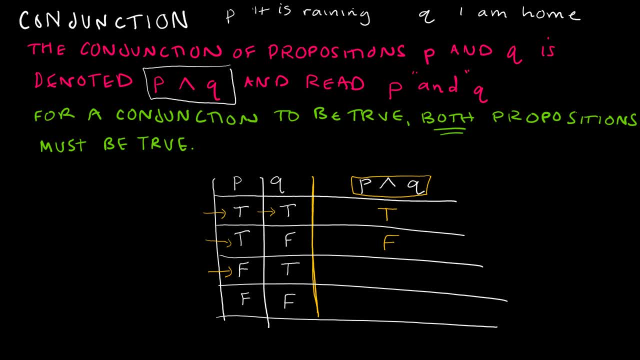 I am home And I am home. So it's not raining and I am home, of course, would still be false, because it's not raining And this row represents it's not rain, raining. I am not home- Again, false, because they both have to. 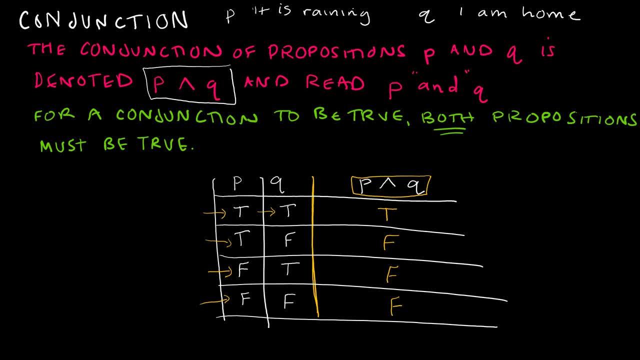 be true, for it to be true. So it doesn't matter if you put these propositions of meaning to the propositions, But keep in mind that that's what you'll be doing quite often is you'll be using those propositions, using those statements, to write them as. 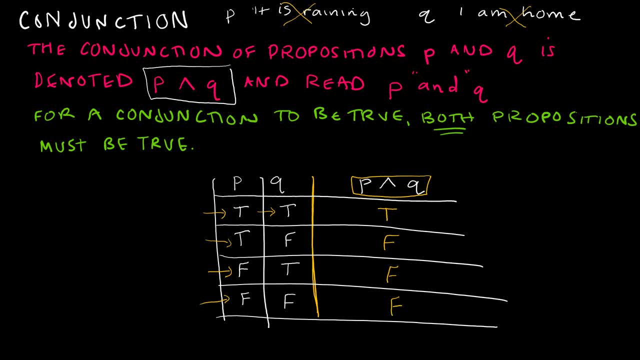 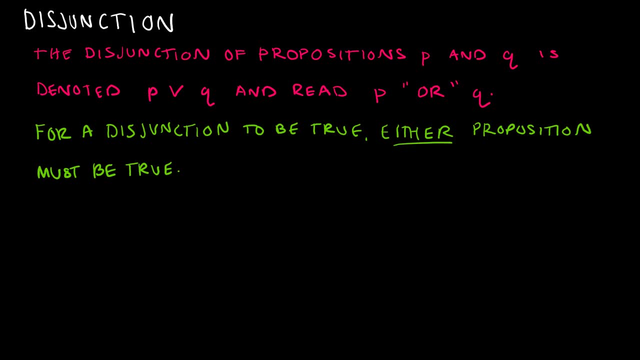 letters and then go from there to make the truth table. Another connective is the disjunction. The disjunction of propositions P and Q is denoted P with the opposite facing arrow. so basically a V and read P or Q And for a disjunction to be 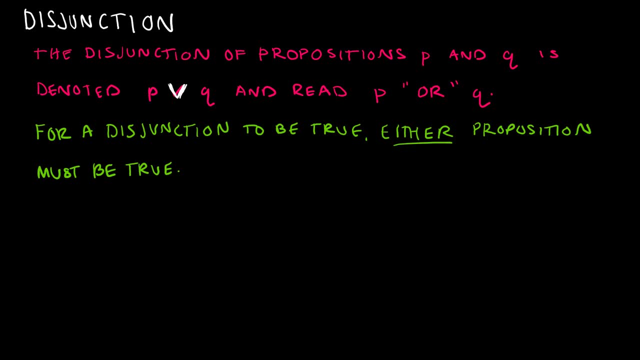 true, either proposition must be true. So when we were talking about a conjunction, both had to be true for the conjunction to be true, For a disjunction to be true, either proposition must be junction, either proposition must be true. so again, when I create my truth table, 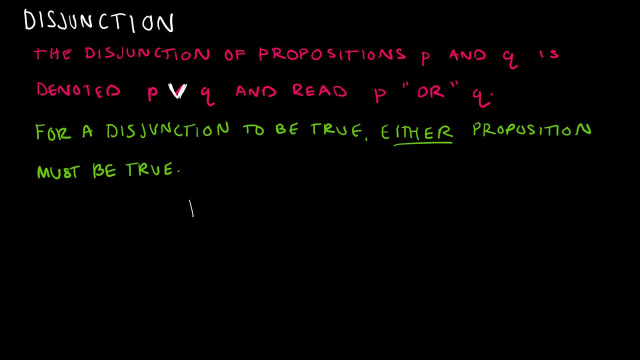 I'm always going to start on that left side where I'm giving all of the different combinations, and on the left side again, I've got true, true, true, false, false, true, false, false. so that's just the combination side. I haven't done anything yet. on the right side is where I'm going to write, whatever my results. 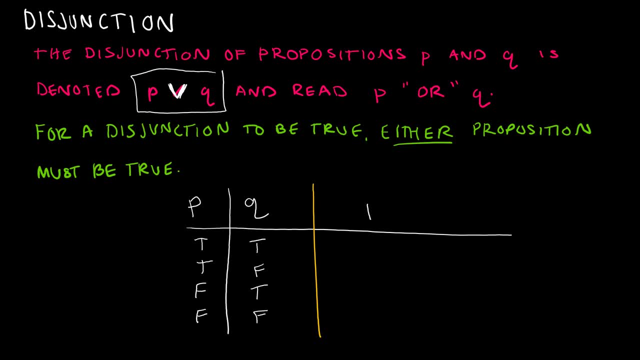 are. in this case, the connective is the disjunction, so I'm going to write P or Q, and again I think of a disjunction, or the or, as being a cup. so if you can put anything in the cup, if either one is true, then the result is true. so 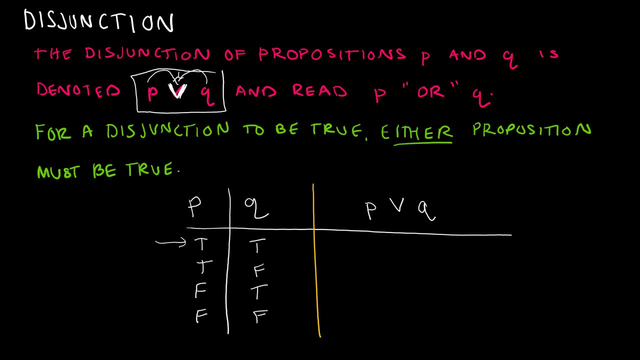 you know, if P is true and Q is true, then P or Q is true, because either one of them is true. if P is true but Q is false, P or Q is still true because P was true. only one of them needs to be true. they can both be true, but only one of them needs. 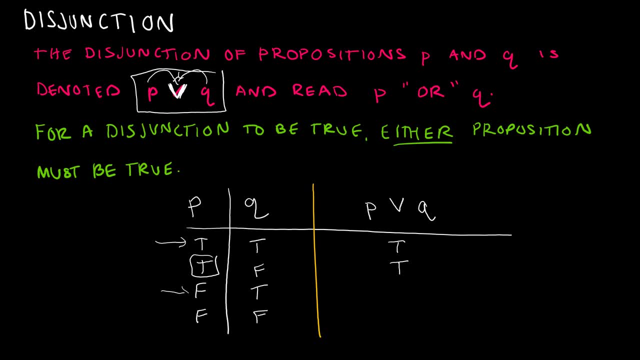 to be true. if P is false but Q is true, p or q is still true because q was true. So the only false value I'm going to have is where both p and q are false, because neither one is true and for the disjunction to be true. 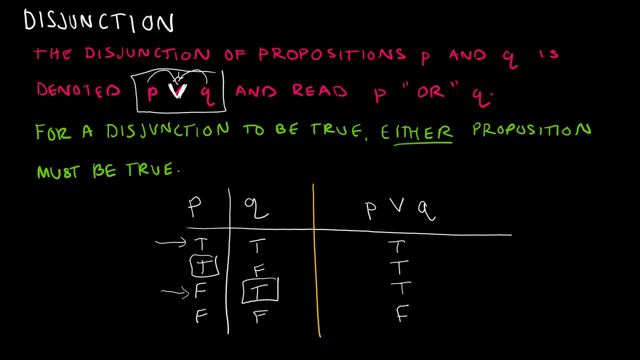 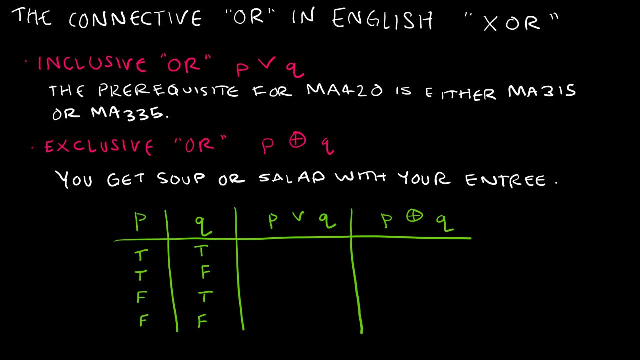 either proposition has to be true, So that's my solution. The ors can get a little bit tricky. Most of the time in mathematics we're using that inclusive or that we just talked about. That's the p or q, and that is saying, for instance, the prerequisite. 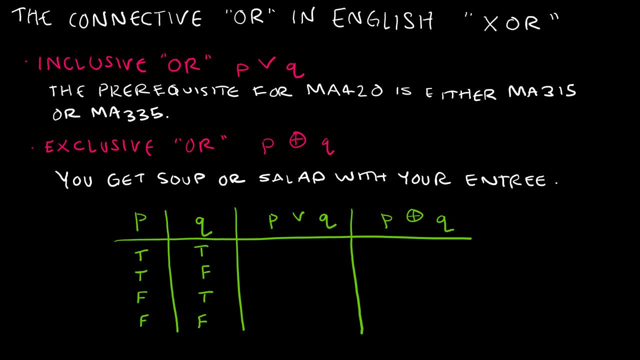 for MA420 is either MA315 or MA335. And by that I mean you could have passed MA315,, you could have passed MA335, or you could have passed both of them and you can still get into MA420. That's the inclusive, or That's the one we use most often. There's also the connective or. 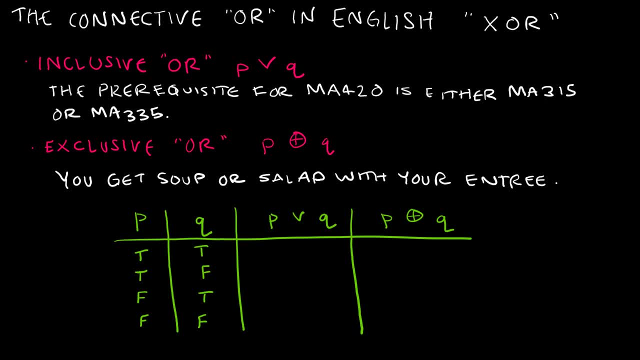 that we use most often. There's also the connective or that we use most often. There's also the in English, which is called XOR, and that is something like: you get soup or salad with your entree. Now, if I'm buying an entree, that means I can get soup or I can get salad, but I can't get. 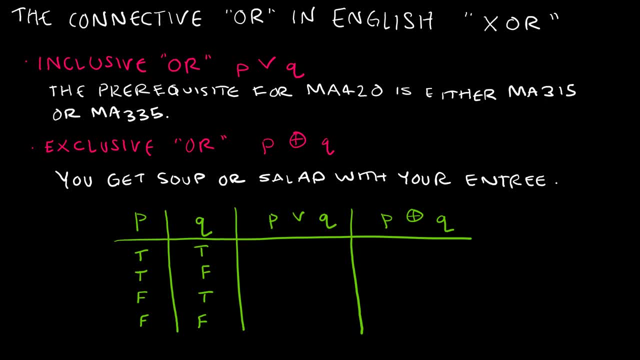 both. I mean I can. I can just pay extra, but I can get one or the other, but I cannot get both. So while we just finished talking about the inclusive or where we said: if either is true, then it's true, And that was.